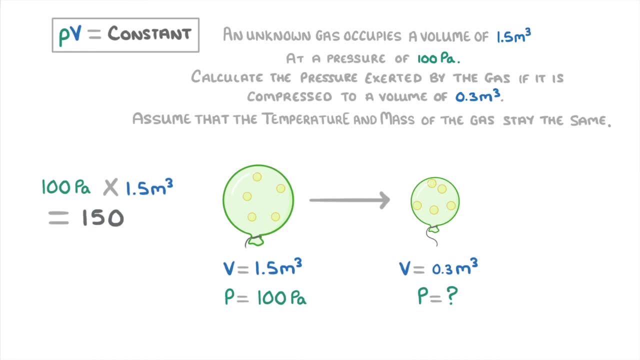 Then, looking at our other gas sample, we know that its pressure times, its volume, must also equal 150.. So to find the pressure we can just plug in the 0.3, and then rearrange by dividing both sides by 0.3, which gives us 500 pascals. 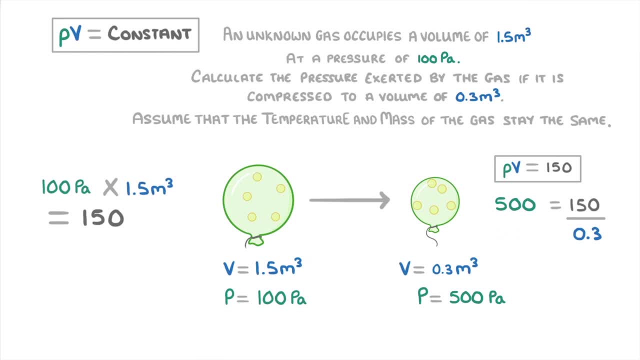 We know that this new container must be at a pressure of 500 pascals. Now there is another way of doing this that some people prefer, Because the constant is the same for both containers. instead of actually figuring out the constant, we can just say that the pressure times the volume in the first container equals. 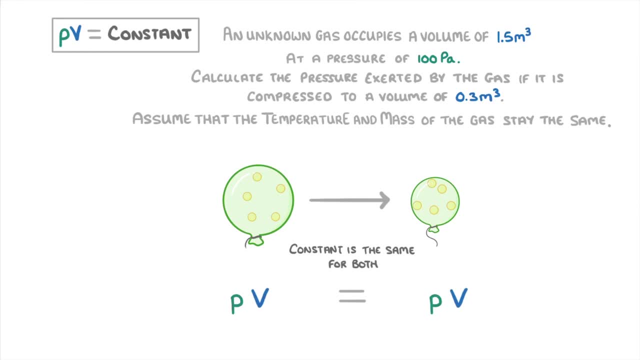 the pressure times the volume in the second container. And to avoid getting the numbers confused, we normally say that P1 times V1 equals the P2 times V2.. So 100 times 1.5 equals something times 0.3, which we can rearrange to get 500 pascals. 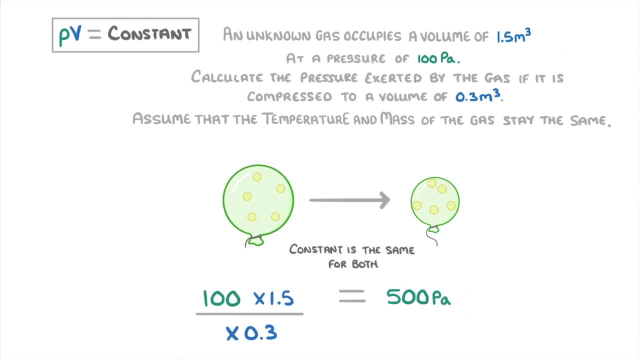 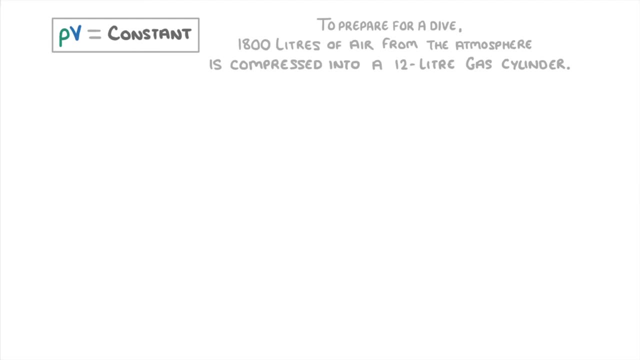 just like we got before, Let's try one more. To prepare for a dive. 1800 litres of air from the atmosphere is compressed into a 12 litre gas cylinder. Calculate the pressure of the air in the cylinder. Assume that the temperature remains constant and that atmospheric pressure is 101 kilopascals. 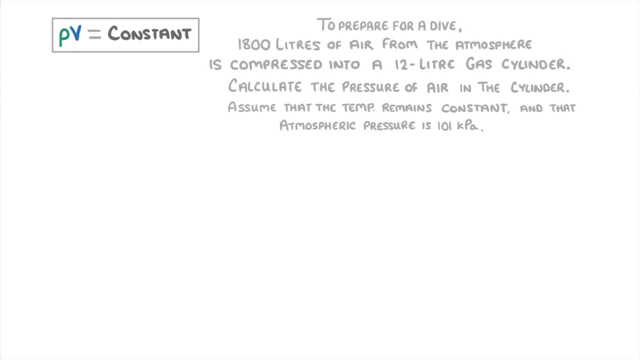 In this question, it's a bit more difficult to see which values we're meant to use, where We're basically taking a volume of 1800 litres of atmospheric air and compressing it into the much smaller volume of 12 litres at an unknown pressure. 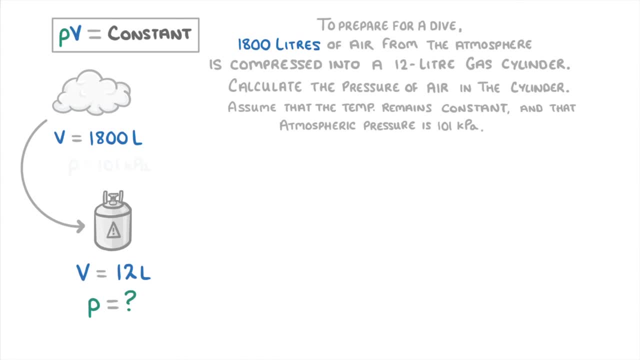 The key thing to notice, though, is that atmospheric air will have a pressure of 101 kilopascals, So, if we take the equation we just mentioned, all we have to do is substitute in 101 times 1800, which will equal something times 12.. 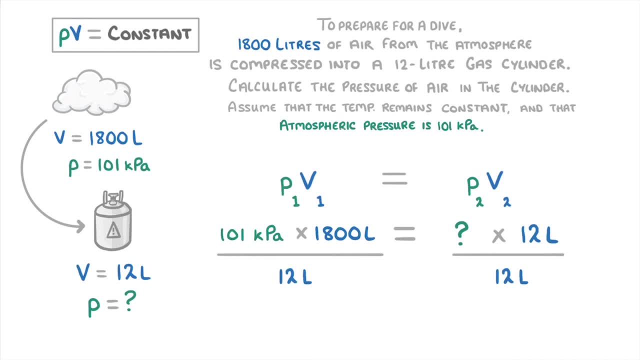 Then we just divide both sides by 12, and that'll give us a pressure of 15150.. And, importantly, we can just add in the pressure of the air, which will be something times 12.. And then we just divide both sides by 12..